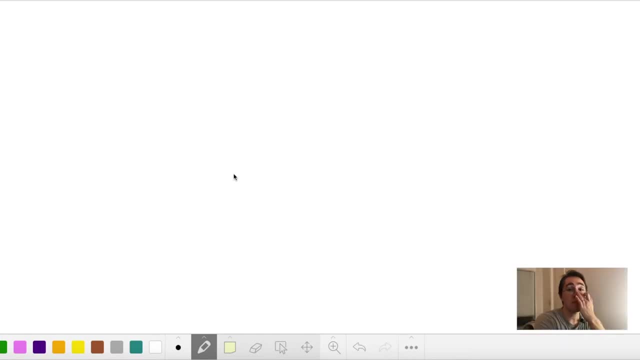 Hi. so I wanted to talk a little bit today about the famous n choose k formula. So n choose k should be equal to n factorial over n minus k factorial times k factorial. And what I found when I first was introduced to this formula, I would always find that this 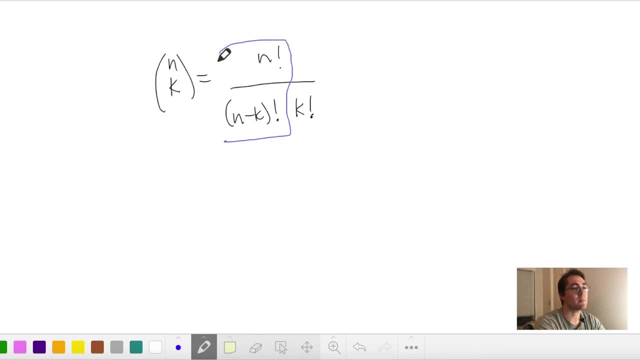 part was fine. I was okay with this part of the formula. So this n factorial over n minus k factorial, we know that. that is the number of ways of choosing k objects from n where order matters. Yep, Okay, the part that was always not necessarily confusing, it was always. 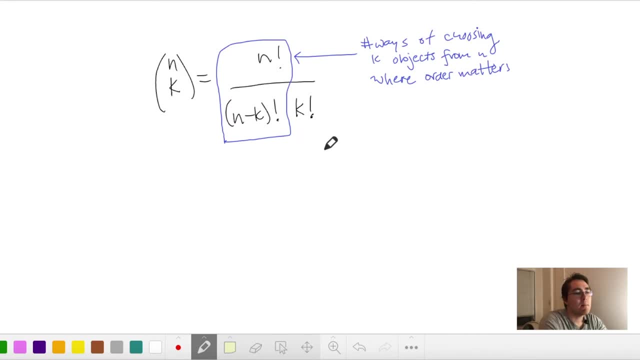 you know, in some respect intuitive but hard to see exactly where it came from. was this k factorial factor? Now, most of the time I think this was sort of explained away with an aside, something like: and then you just got to divide out by the permutations, right, And that's all well and good. 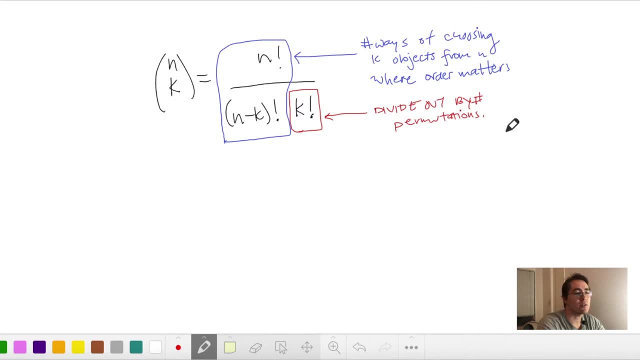 Like I said, it's not necessarily that it's super counterintuitive or weird or anything like that. It makes sense. But you know where exactly is this coming from? How exactly do we get this k factorial, For example? if I'm dividing out by it, well, when was I multiplying by it? 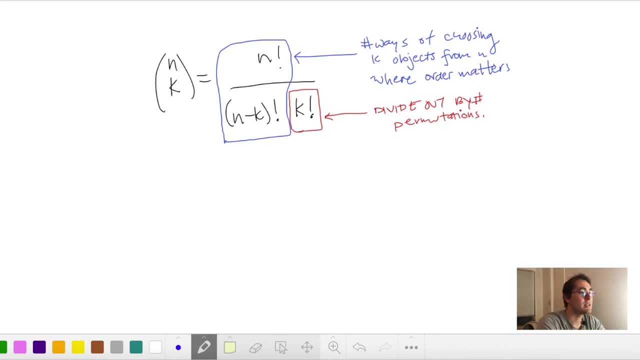 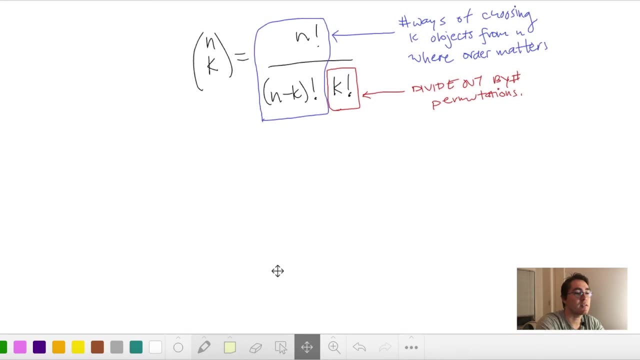 right, And so actually to make this crystal clear, it's maybe a lot easier than younger me might have thought, But literally I think it's. it really comes together when you write the formula this way. Ah, so much nicer, Yes, And if you can already see the logic behind this at this point, 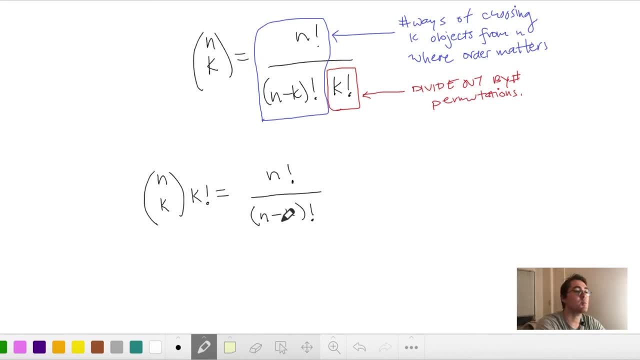 I mean you can just turn this video off And we're done, Because at this point I think this way of writing the formula it it makes a lot more sense. So once again, we already know what this side of the formula represents. We know that that is just the number of ways of. 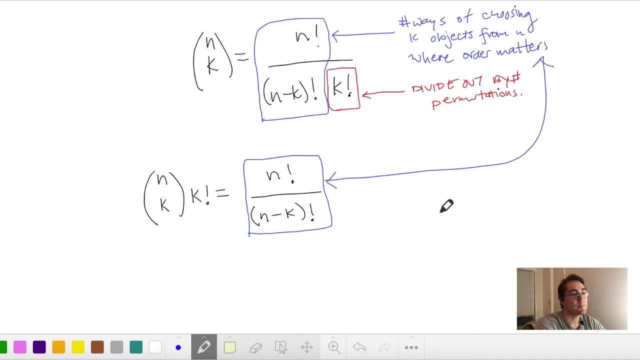 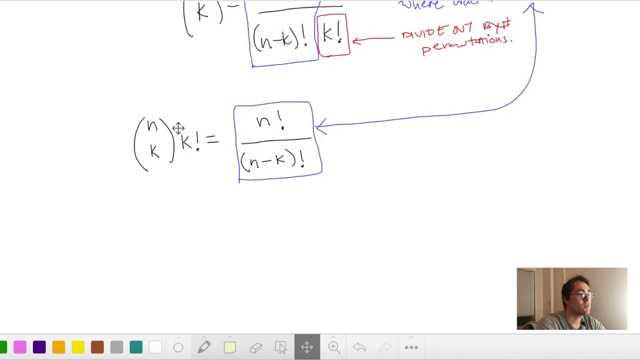 selecting k objects from n where order does matter. Now just to kind of you know, really hone this in here, this side of the formula, let's suppose that we don't actually know yet what n choose k is. We don't know the formula for it, I should say yet right. But conceptually we know that this is the number of ways of choosing k objects from n where order doesn't matter. 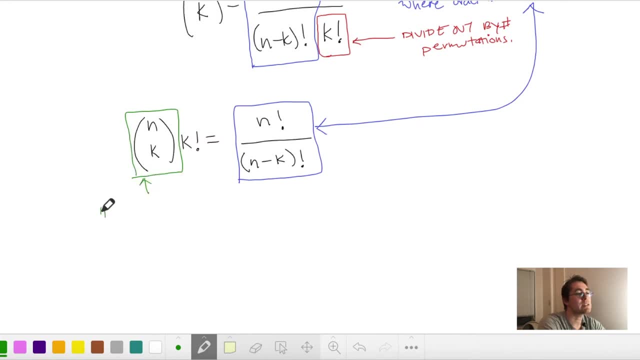 But conceptually we know that this is the number of ways of choosing k objects from n, where order doesn't matter this time around um and, if you want, like a slightly more rigorous definition, right, because this all feels very um sort of physical, like you know, bob, from you know wherever is asking for this. 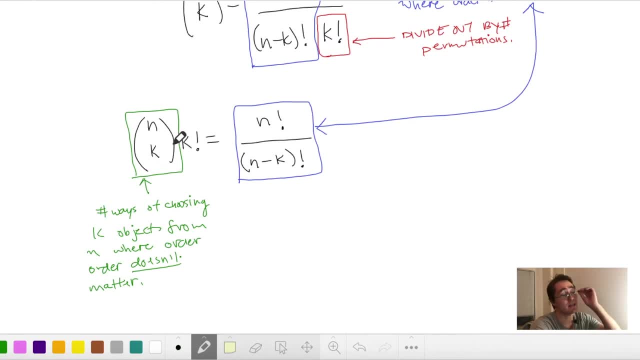 or something, but you could also think of this then, as the number of um k element subsets of an n element set. right? but anyway, going back to what we were saying, this is where order doesn't matter, right, it's the same concept. from n we're selecting k objects, but this time we don't care about the. 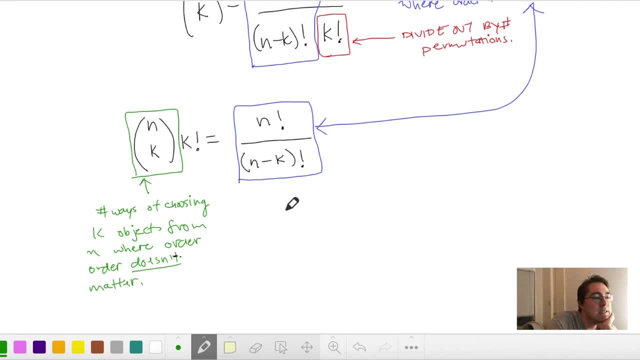 order. okay, just to kind of illustrate, you know what's going on here. we could say: let's suppose we had this set: one, two, three, four, five, right? and let's say i'm picking three elements at a time, right? so let's say i had this set. 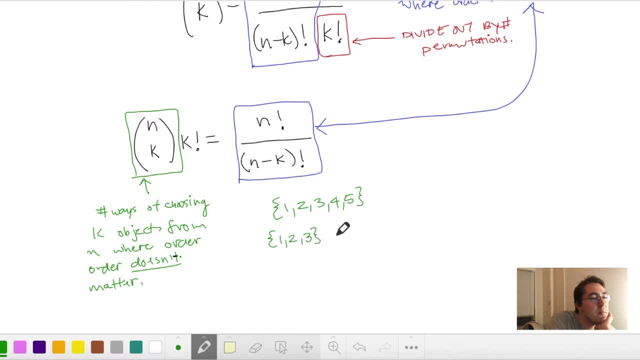 one, two, three. for me, if i don't care about the order, that's the same, as you know. say two, three, one, and uh, um, three, two, one, and so on and so forth. there's lots of different ways of rearranging this, but to me these are all going to count as just one right. these only supply one to the count. i really 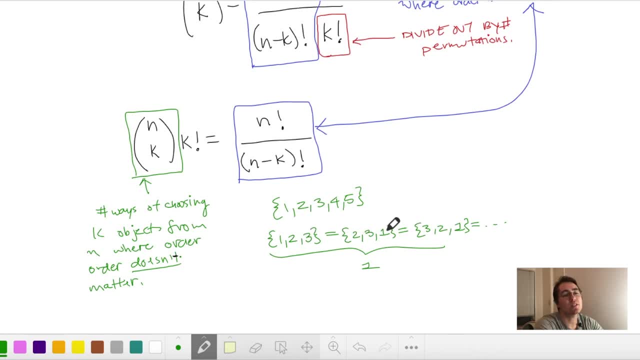 don't want to count this multiple times because, although the order is different in each one of these, they're different. in each one of these they're different. in each one of these they're the same elements. It's a 1, a 2, and a 3.. A 1, a 2, and a 3.. And, like I said, I don't really care. 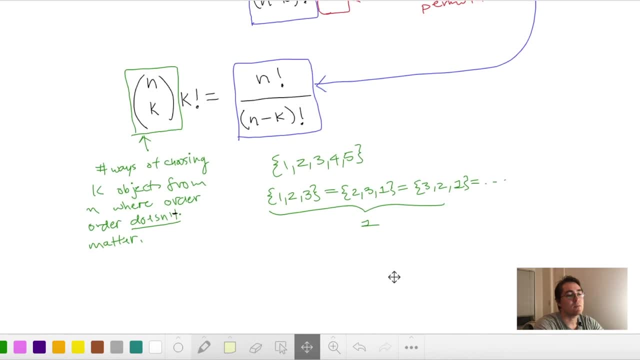 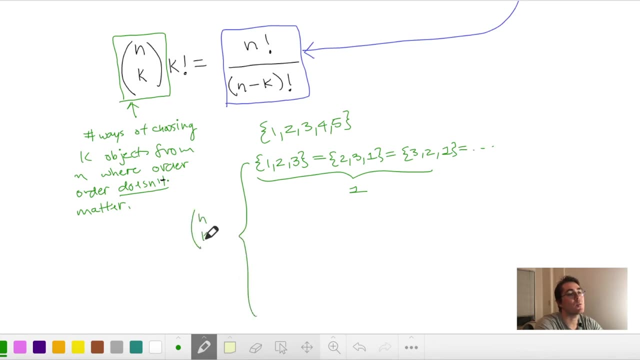 about the order, And now we see that the number of ways of doing this is n choose k, right? That was how we in some sense defined it. n choose k is just the number of ways of doing this. So there might be another way of doing this. Say, maybe I pick 4,, 2,, 5, right? That's just another. 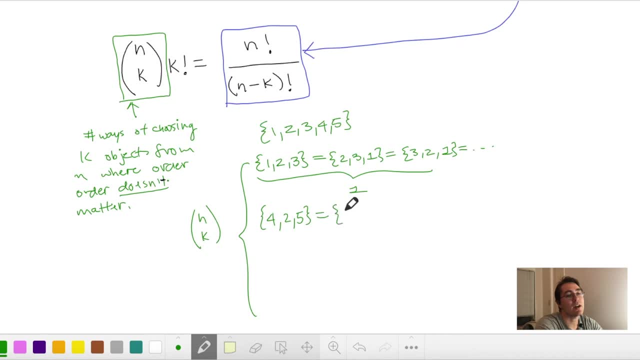 way of doing it right, I could write that as 5, 2, 4.. But again, these are just equivalent to me. What's not equivalent are these up here right? 4, 2, 5 is very different from this one. It's. 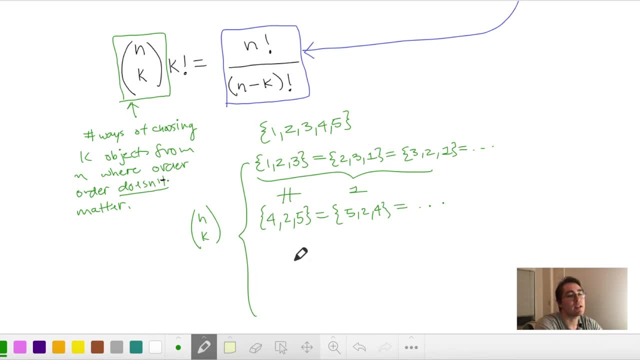 different from that one, It's different from these. They're all very, very different, And I can keep doing this, But, with that said, if I enumerate all the way down, I'll have n choose k of these ways of doing things And you. can think of this as a number of ways of doing things, So I'll have n choose k of these ways of doing things, And you can think of this as a number of ways of doing things. And you can think of this as a number of ways of doing things, And you can think of this as a number of ways of doing things. 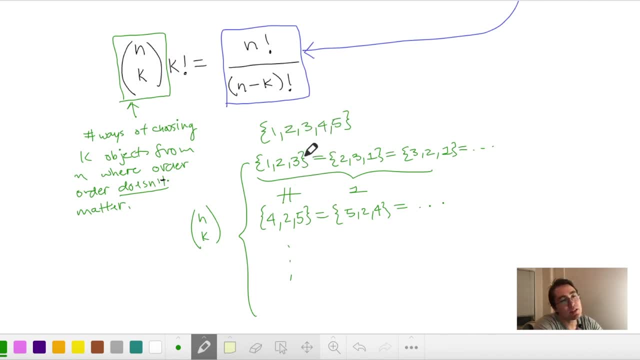 sort of like unique selections From this collection of three elements from this set. there is at least one element in here that's not in there, right, Because these are not going to just be reorderings of the same thing. right, And that's true as I go down vertically. But 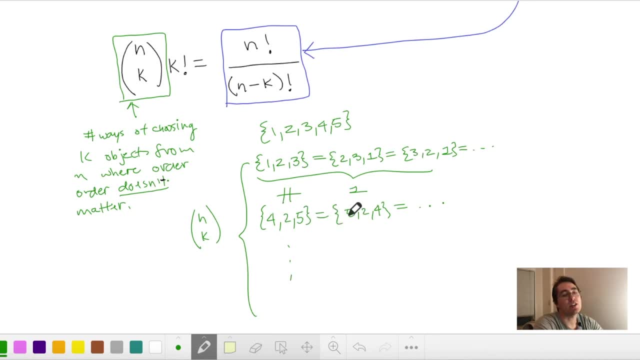 horizontally in each one of these. it's just a rearrangement of the same elements. I'm just permuting them right And so, with that said, this is sort of the number of ways of uniquely selecting three elements right, And there's n choose k of them. But what if I did care about? 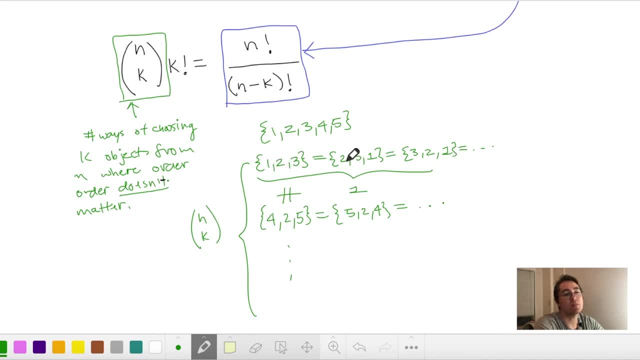 order. now What if you know? for me, 1, 2, 3 was different from 2, 3, 1 was different from 3, 2, 1.. I want to start actually counting these, Like this would be 1,. this would be another 1,. 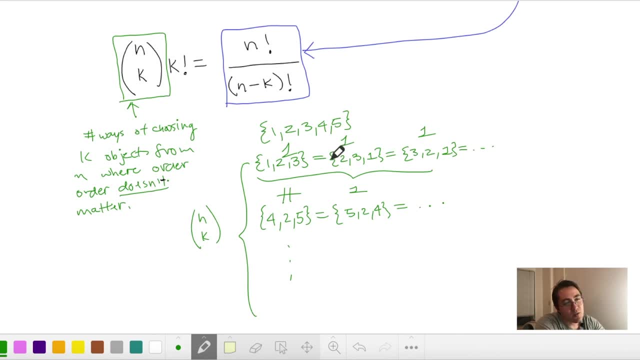 this would be another 1, and so on and so forth. Well, if I did that for this entire choice, sort of you could think of this in some sense, if you want, as if you take the set of tuples- three tuples here- from this set. In other words, we're ordering them in this set. 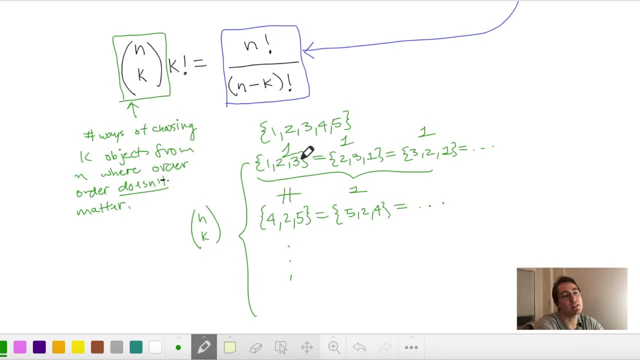 Order matters. You could think of this as almost like an equivalence class right, The equivalence relation here being that they have the same elements. You could actually show that that's an equivalence relation. if you know that's something that you want, if you wanted to make. 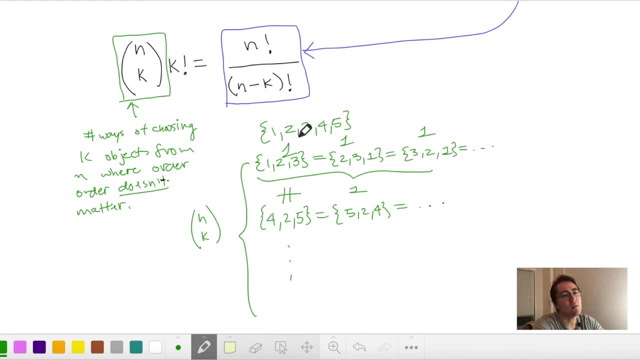 this a little more rigorous. But in any case, what if I care about the order here, these permuting, changing the order of these things? Well, we know that since there's three elements here, there's going to be three factorial, And to generalize that would be k factorial. 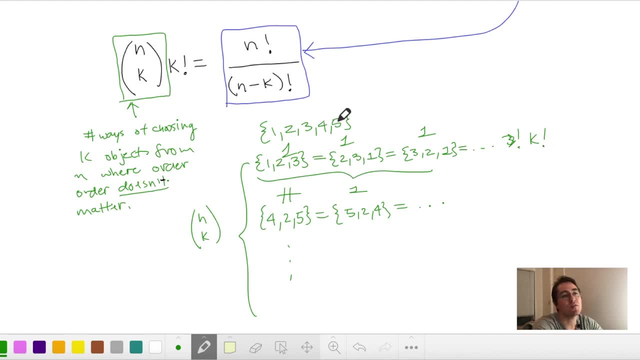 If, instead of picking three, I was picking four, and instead of this being five, it went up from 1,, 2, all the way up to n right. So, from the n, from the n, I'm picking, k, Picking. 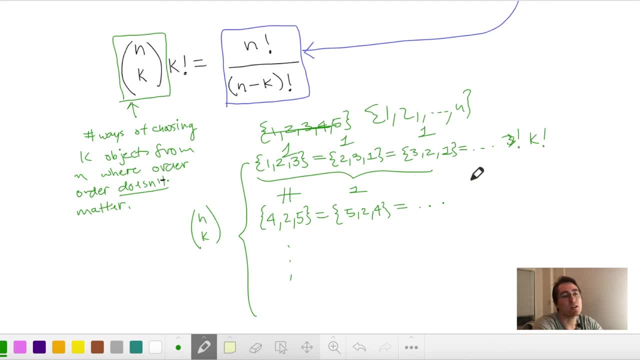 k. in this case it was 5 and 3. So it's k factorial here. And that will get me all the ways of selecting these numbers: 1,, 2,, 3, and all of their permutations, In other words. 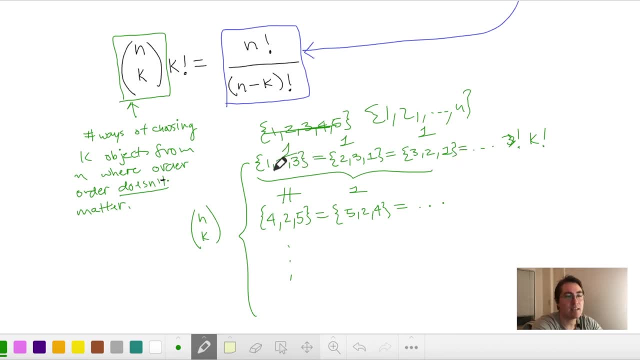 it's really all the ways of selecting this particular collection where order does matter, All right, And I could do that for down here as well, k factorial, And I could keep doing that over and, over and over again for all of these, For each one of these unique selections. 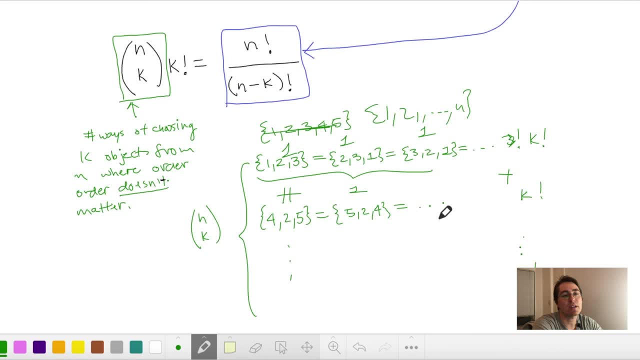 I'll sort of keep permuting them and counting those permutations and I'll get k factorial every single time And if I add them all up, k factorial plus k factorial plus and so on and so forth, plus k factorial. let's see what I did. How many of these were there There? 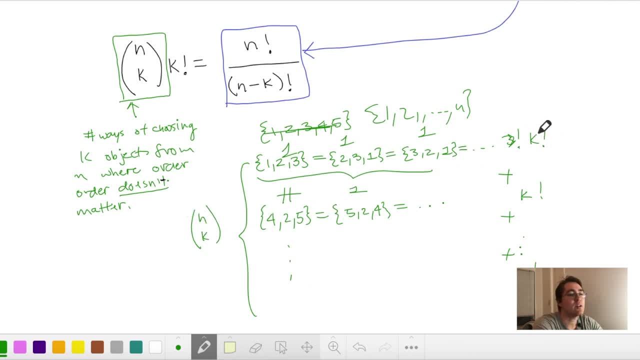 were n choose k, And I'm adding k factorial that many times. So that's n choose k factorial, choose k times k factorial. But now look what I actually have over here. I have all the ways of picking 1, 2, 3 and its permutations, All the ways of picking 4, 2, 5 and its permutations, And 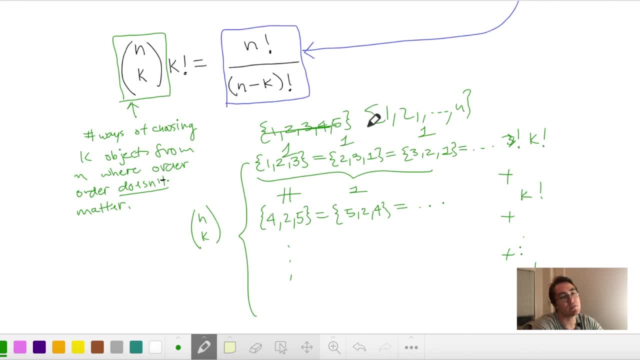 I'm doing this for each unique selection of three elements from my set. In other words, when I'm doing this, adding up all the k factorials, what I'm really saying is all the number of ways of picking k elements from n, where order does matter. Ah, but we already said we know what that is. 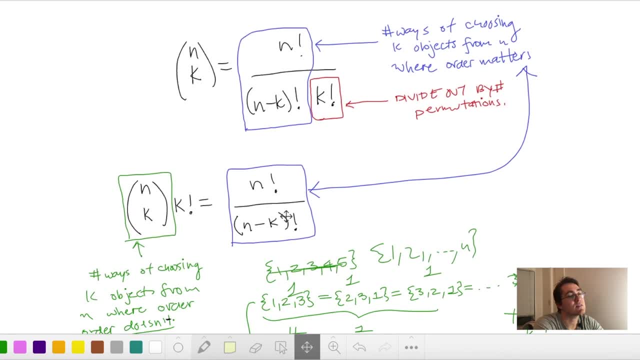 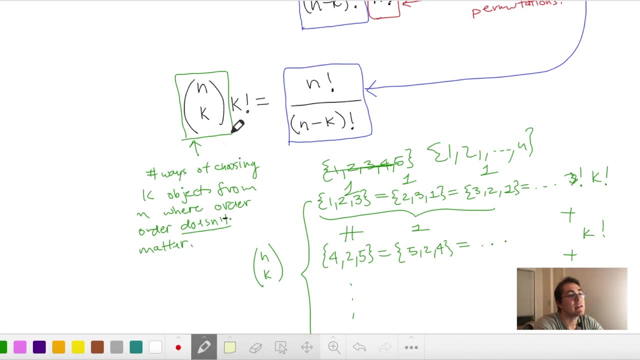 Number of ways of choosing k from n where order does matter. That's this right here, And that's really all there is to this formula, because now you can just divide out by this k factorial, which was, I guess. that aside, that maybe I was just too dumb to realize, But this is where the